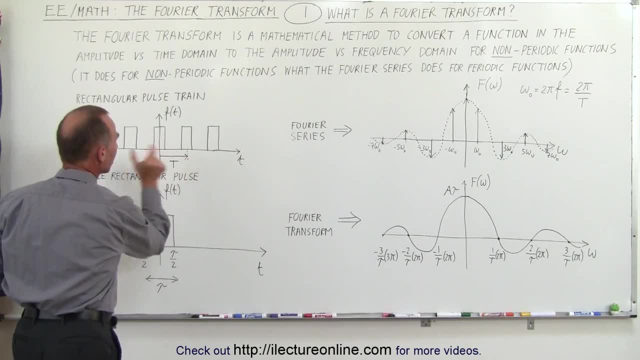 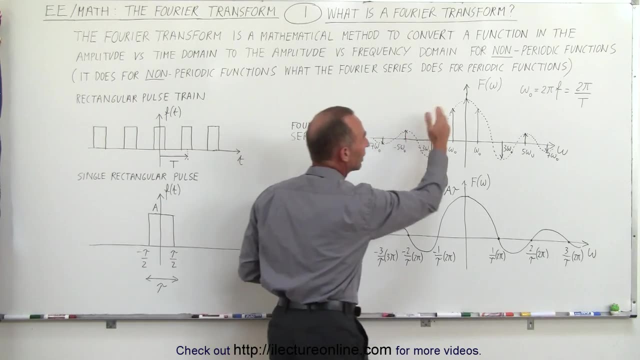 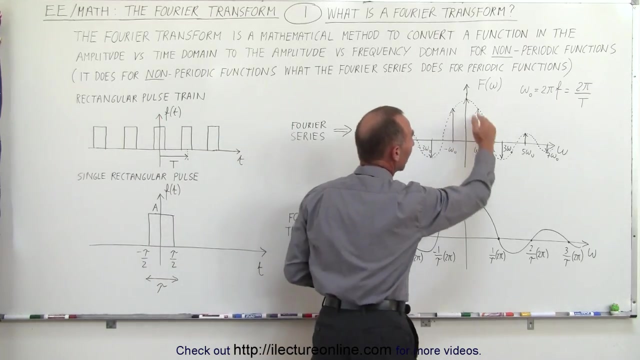 Fourier series of that. notice that this here is the period, this is the amplitude in the time domain. right here we do Fourier series and we get the amplitude in the frequency domain and notice that if it's centered about the central vertical axis, then we get something that looks like a sinc function. notice that Omega sub naught. we're going to start. 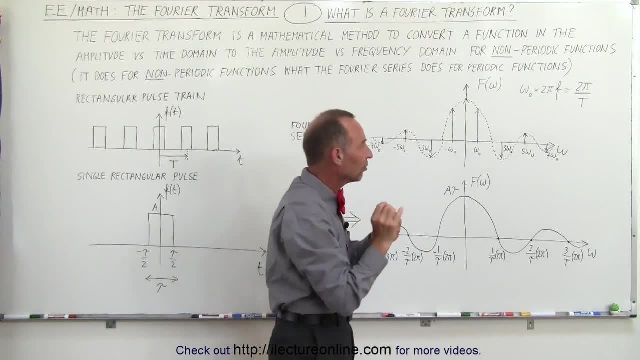 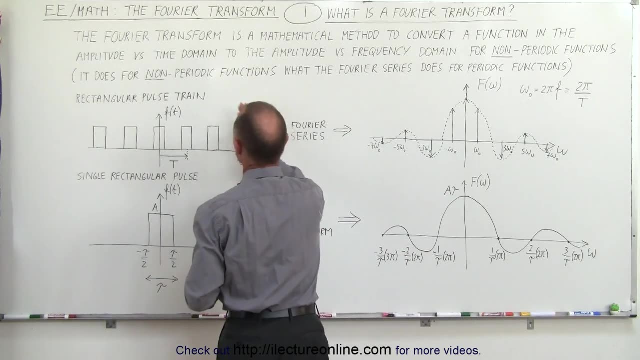 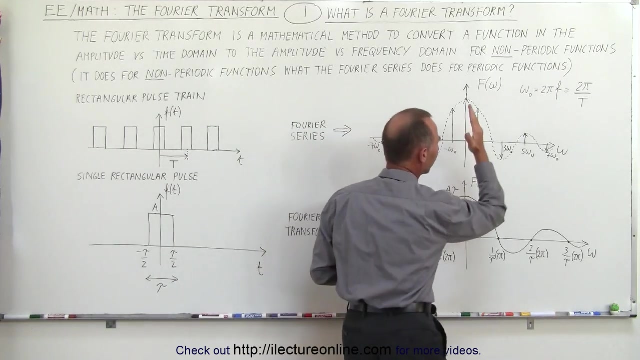 using a sub naught here, because we have discrete frequency values. those discrete frequency values are where we find amplitudes for the Fourier series, which is the Fourier series translation of the time domain function. notice for specific frequency values. we have specific amplitudes and we do not consider anything in between. we have what we call the 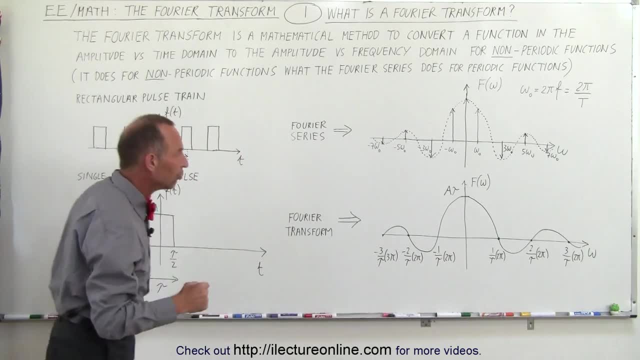 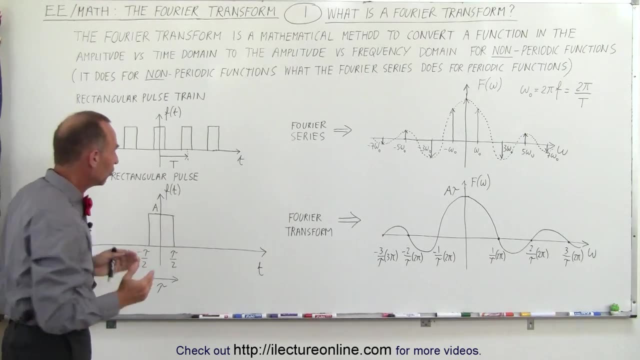 Fourier series and we would consider anything in between and what we would consider the Fourier series. that's what I call the Fourier transform, and this has all these discrete values here, and when we take the Fourier transform, notice we do that for a single pulse, so instead of having a whole, infinite 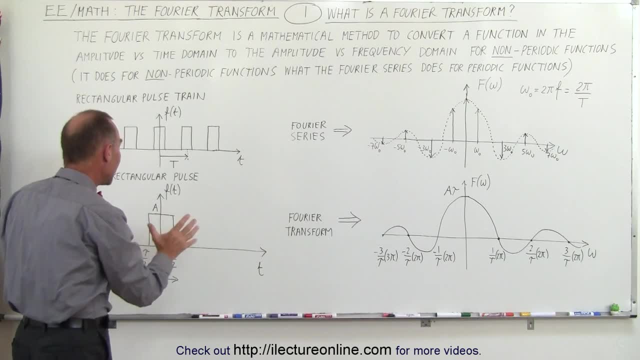 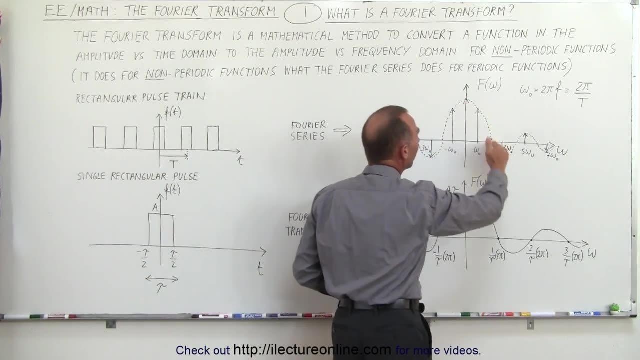 train, basically of pulses. we just take a single pulse. and now we want to do the same thing. we want to find the frequency versus time domain function of this. that's what we call the Fourier transform. notice, if we draw a dotted line about the amplitudes of these discrete values, when 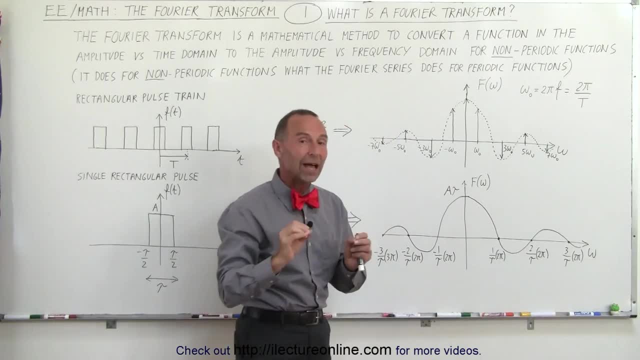 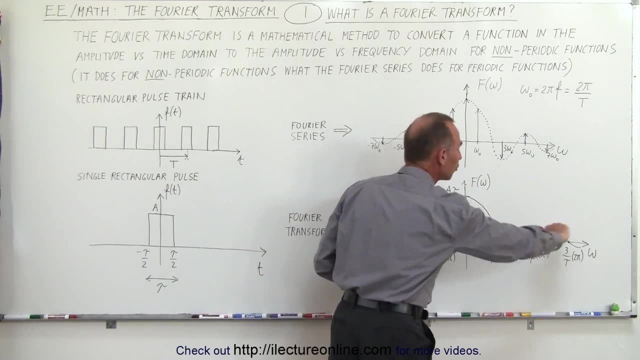 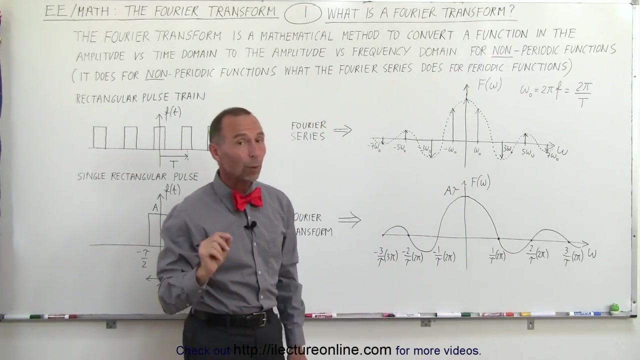 that same type of graph becomes the actual graph of the Fourier transform. Notice: there's no discrete values here. There's just a continuous function that gives us amplitude versus frequency instead of the discrete values. like that, What we do see is that there's places. 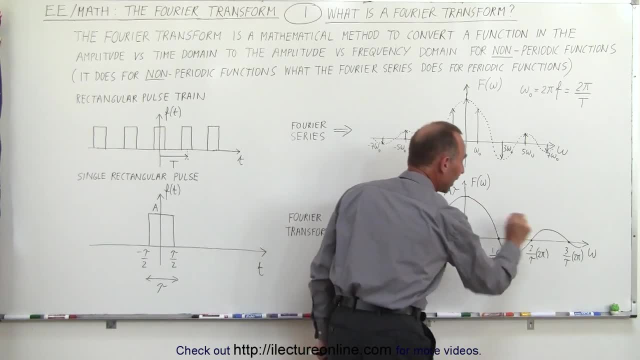 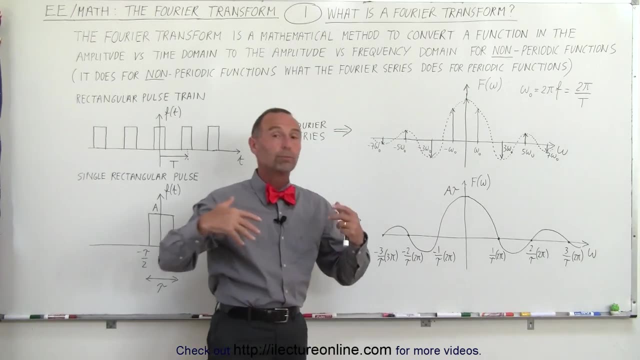 where it goes through the horizontal axis and we can find what those values are equal to. It turns out the values where the function. in this particular case, of course, there's going to be a whole bunch of different kind of Fourier transforms for different kind of inputs. 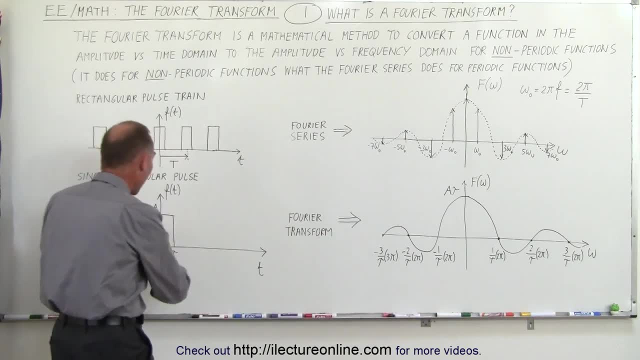 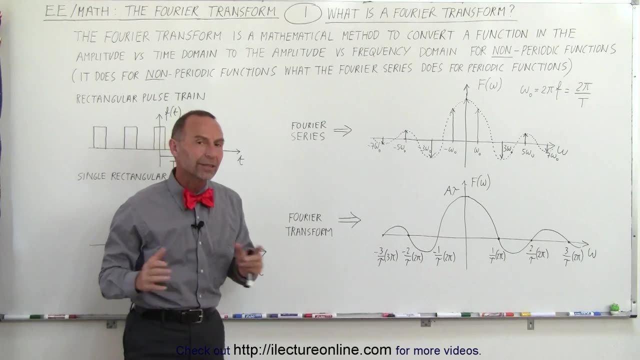 And we'll learn all about that later. And then we'll learn what happens when you widen the pulse, when you narrow the pulse, and so forth, What happens when the pulse becomes infinitely long, things like that, And so we'll see how to do that later. 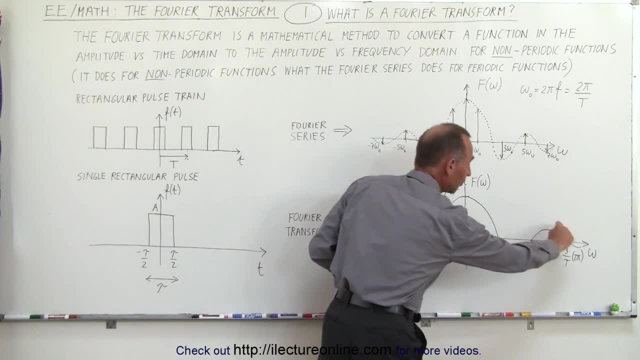 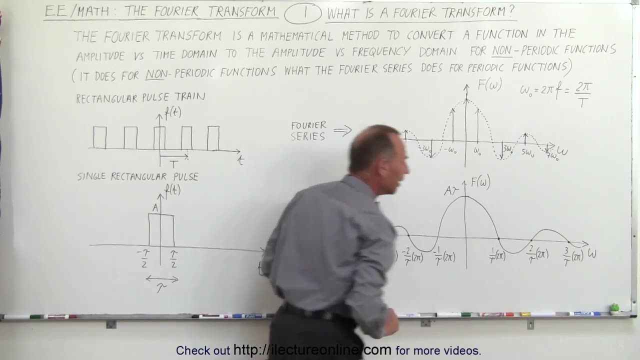 But at this point realize that the place where it crosses the horizontal axis right here, it's one over tau times two pi. That would be the frequency of which it does that. Now, one over tau, hmm, tau is the pulse width in this case. 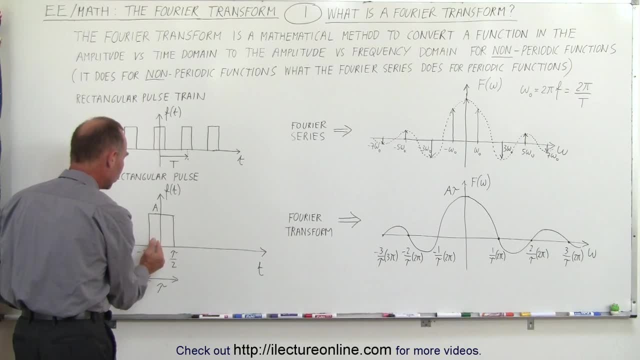 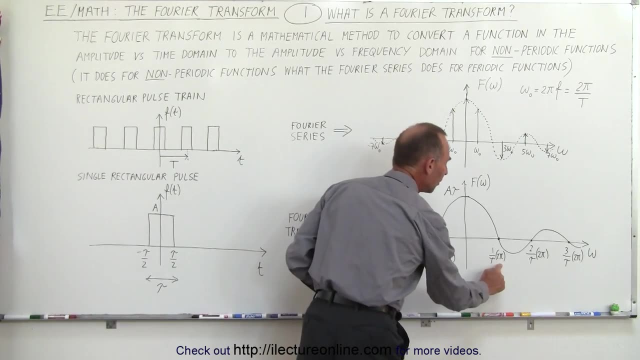 So notice that it goes tau over two to the right and tau over two to the left. So this goes minus tau over two. The total pulse width is tau. And notice that if we take one over tau times two pi, that will be the place right here. 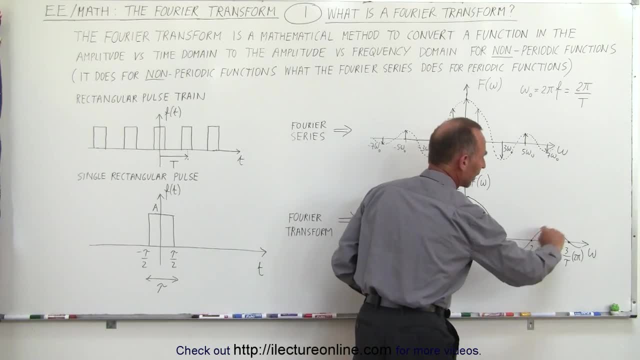 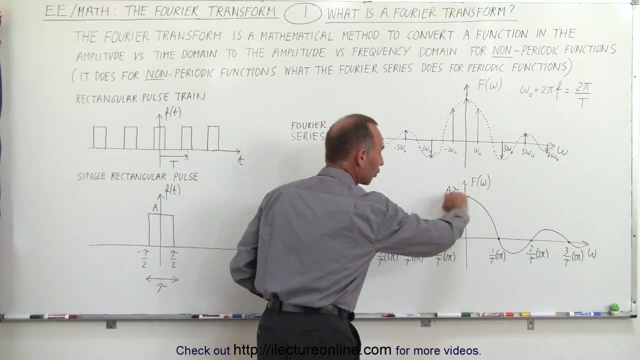 where the function crosses Two over tau times two, pi, where it crosses again three over tau, and so forth. So you can see how that works. The amplitude of the central portion of the curve here is the amplitude of this function. here Let's say that the height here is a, whatever a is. 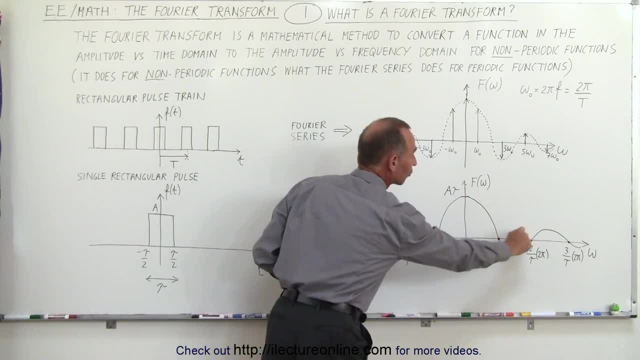 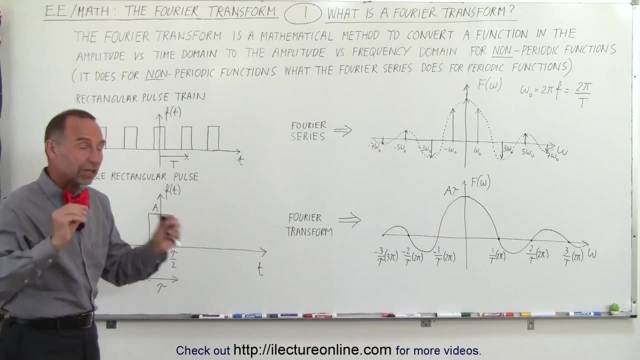 And then we'll multiply that times tau. That gives you the height of the central function here. when we take the Fourier transform, For example, let's say that tau is equal to two seconds. It was a two second pulse centered over the vertical axis right there. 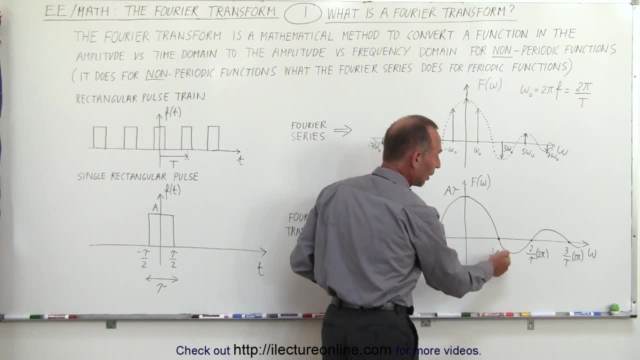 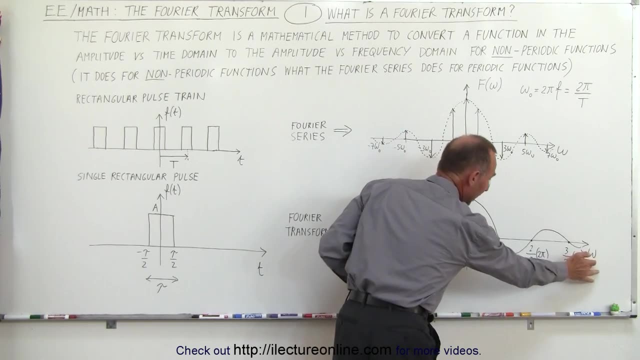 Then we go over here one over two times two. That would cancel out. That means that here the frequency where it goes through the horizontal axis would be equal to, or omega then would be equal to pi, two, pi, three pi and so forth. 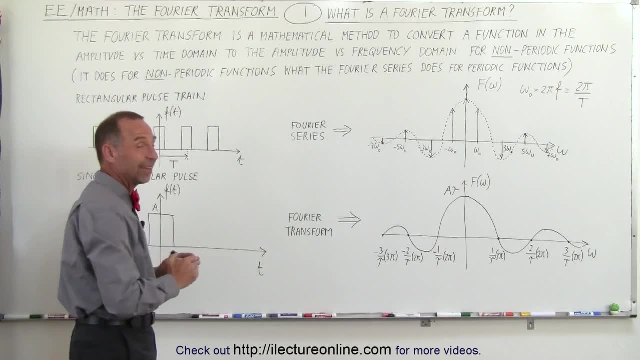 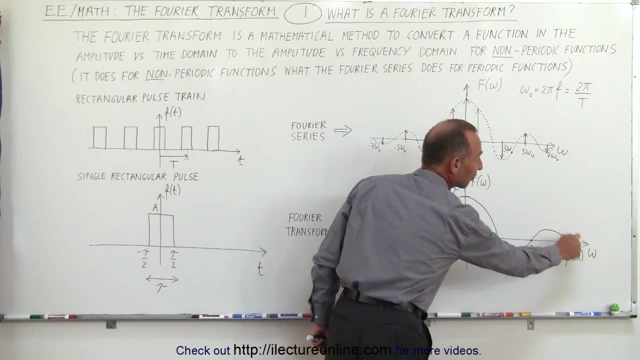 If tau is equal to four seconds- let's say it's wider- then we put one over four, then this would be a half a pi, a full pi, three halves pi, and so forth. And if we narrow the pulse so that this would just be a half a tau. 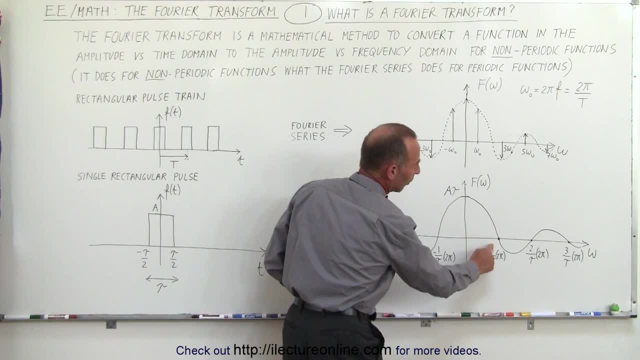 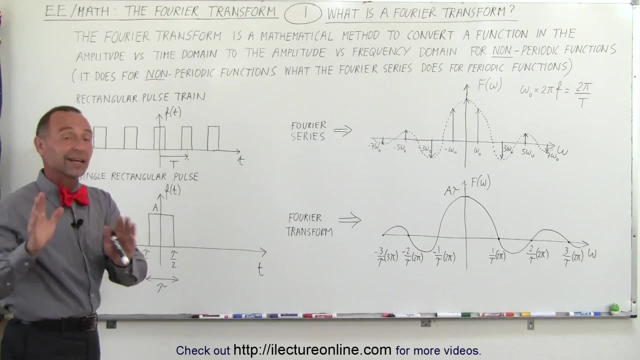 we plug in a half a tau here, then you can see that this would be one half times two pi. Let's see here. Well, that was only one second. There we go, So it was two seconds before We now make it one second long. 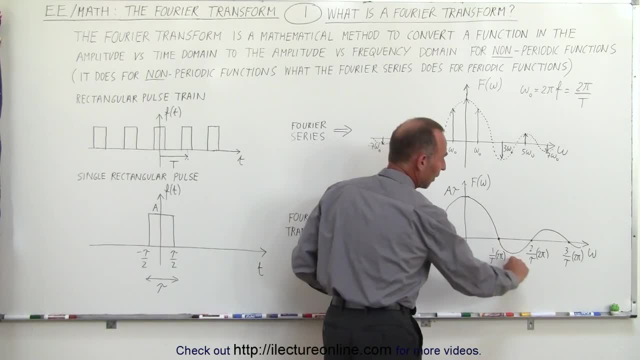 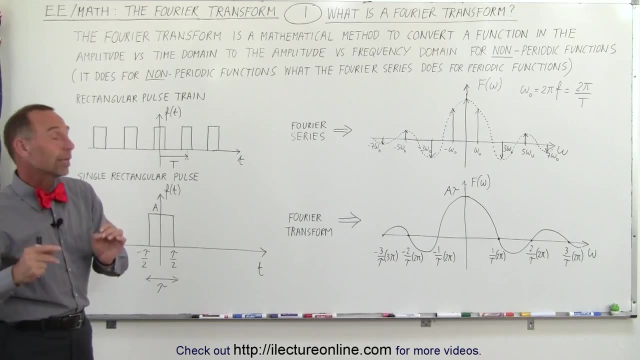 So one over one times two pi. that means the function would go through two pi, four pi, six pi and so forth to the horizontal axis. So you get kind of a feel of how that works. I haven't shown you yet mathematically. 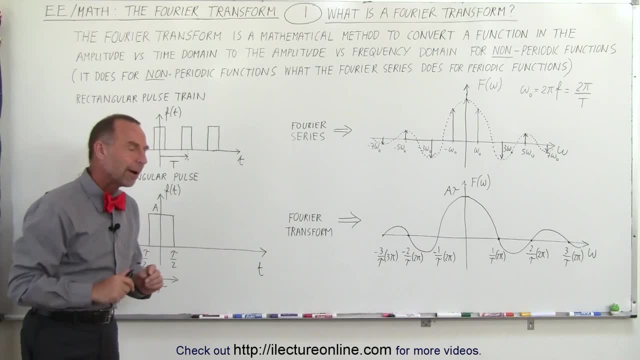 how to do this Fourier transform. That will come on the next video. In the video after that we'll show you some examples, But at least now you have a feel of what the Fourier transform actually is. It always helps to know what you're dealing with. 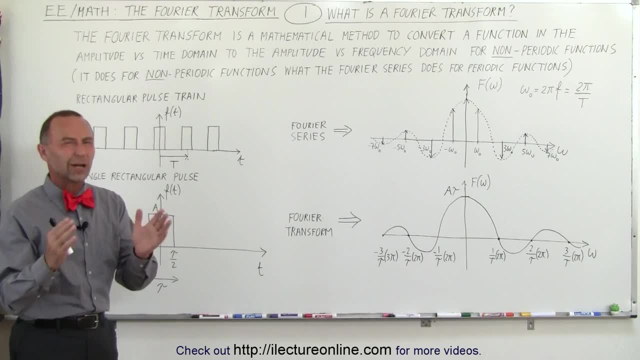 than to start doing mathematical equations and trying to solve these things when you're not really sure what it is in the world that we're doing Now. you know that when you take the Fourier transform, you're basically doing the same thing as taking the Fourier series.